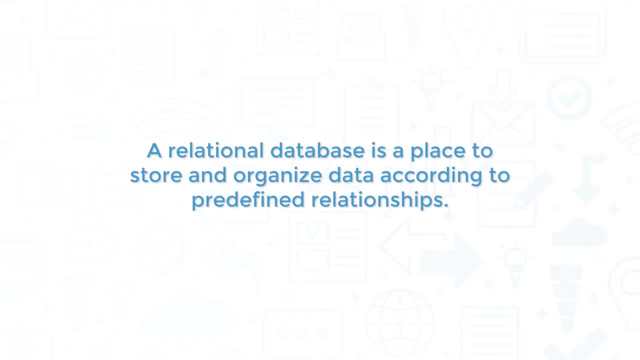 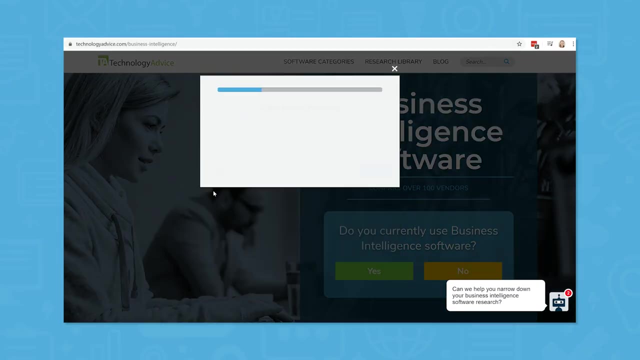 A relational database is a place to store and organize data according to predefined relationships. To learn more about relational databases, keep watching, But if you're looking for a relational database solution, we can help Use our product selection tool at technologyadvicecom to get a. 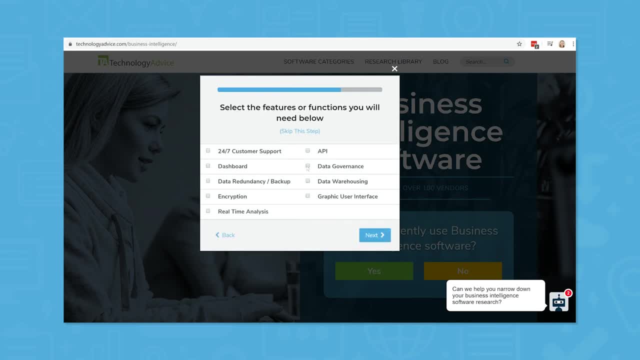 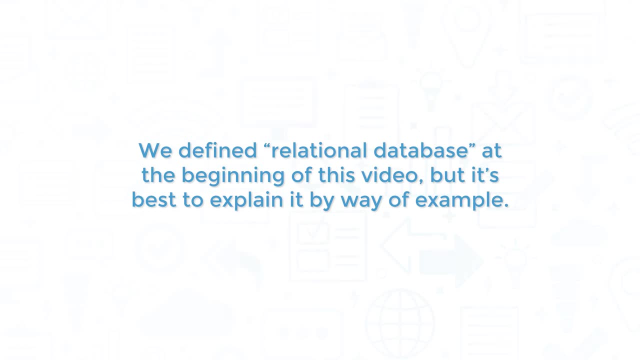 free list of business intelligence software recommendations. Click the link in the description below to get started. We defined relational database at the beginning of this video, but it's best to explain it by way of example. Let's say you own a flower shop. Whenever you take orders for arrangements, 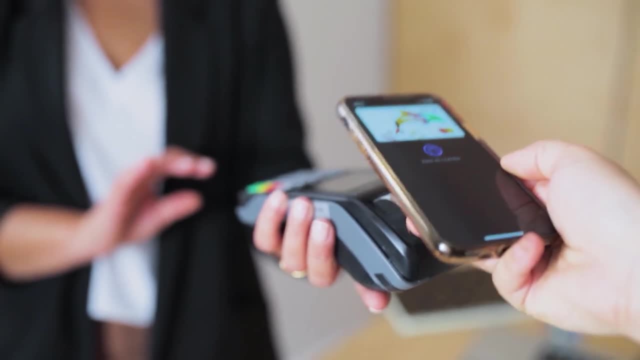 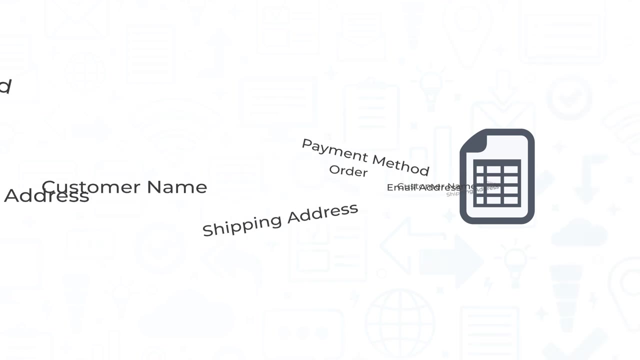 there are several pieces of data. you collect The customer's name, email address, phone number, shipping address, payment method and order. Before you started entering this information in a relational database, you saved it all in a spreadsheet. This worked fine for a little while. 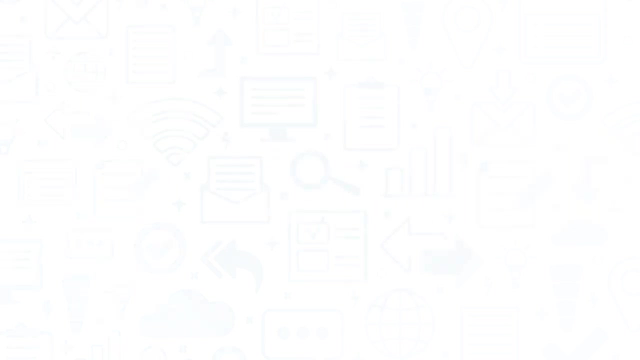 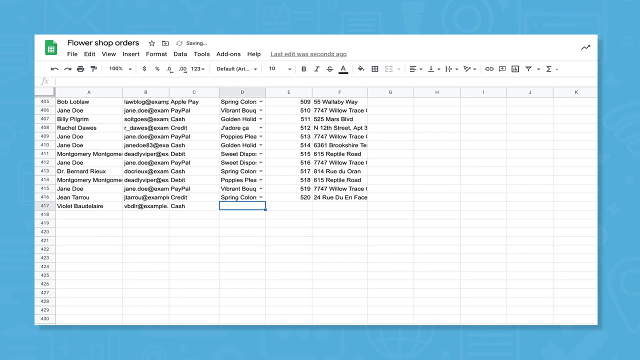 but after you started doing more business, you ran into some problems. First, a lot of the data you generated was redundant, So anytime the same customer placed a new order, you recorded their name, contact information and payment method again and again and again. This created clutter. 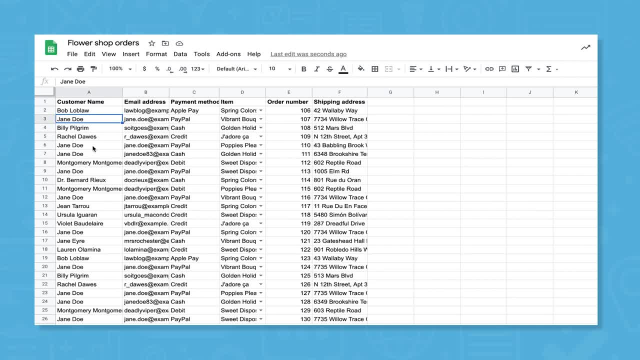 and made it nearly impossible to maintain customer accounts. If you had five different orders from Jane Doe, all with different shipping addresses, it could be tricky to tell her apart from a different person who happened to have the same name. Secondly, spreadsheets weren't very accurate. 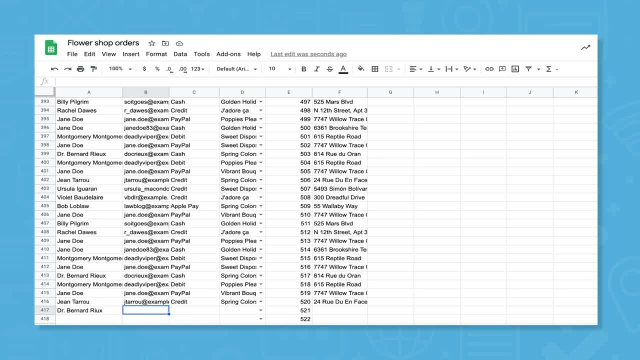 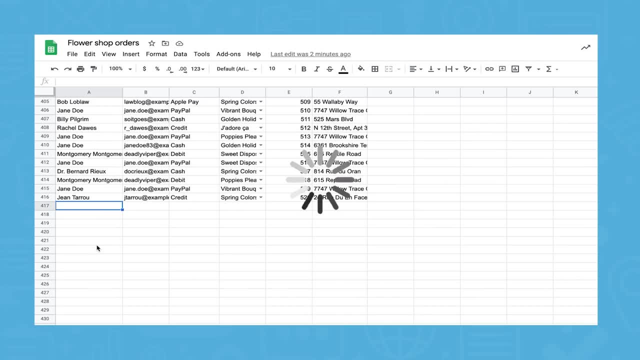 People made typos, and typos caused problems, like the times you accidentally charged one person for an order someone else placed Third. you generated a lot more data than you anticipated. Not only did this slow down your spreadsheet application, but it also made it difficult to ask questions of your 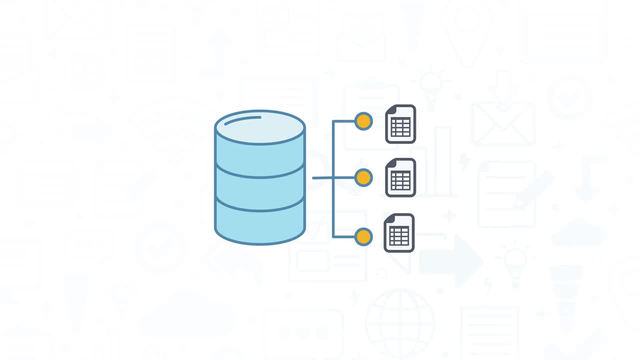 data and generate reports and emails. You also had a lot more data than you anticipated. You also had a lot more data than you anticipated. After noticing the problems you ran into with spreadsheets, you decided to move the orders for your flower shop to a relational database. 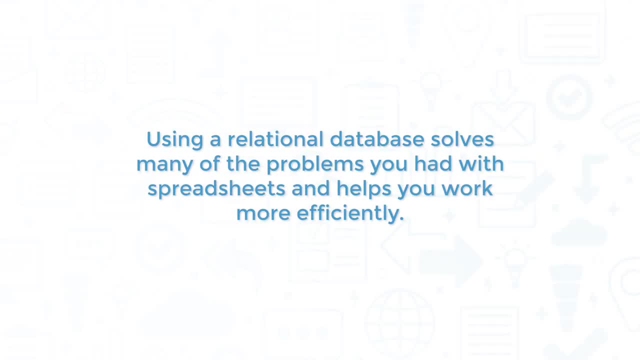 Using a relational database solves many of the problems you had with spreadsheets and helps you work more efficiently. First, the relational database eliminates redundancy through a process called normalization. Normalization lets you move separate data points into their own tables and consolidate duplicate pieces of data.